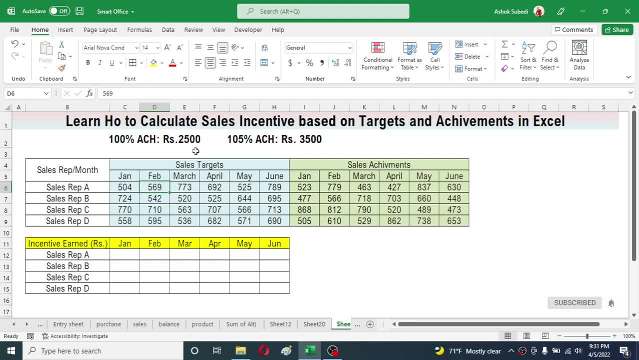 105 percentage of given target, then he or she will be applicable for 3500 monthly incentive. so based on these two criteria here in this table, i need to calculate the incentive earned by these sales persons, and here i am also calculating the grand total incentive earned, which will be calculated by simply using some formula here the major formula we are going. 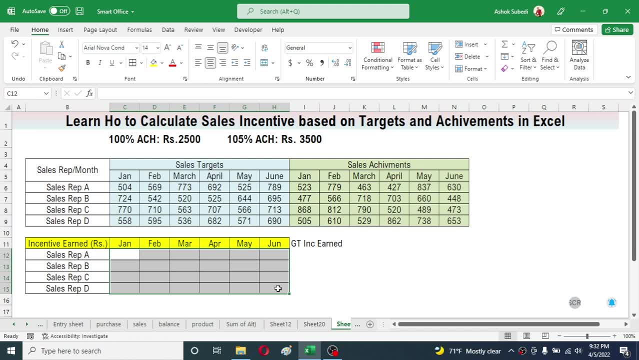 to use. here is the month wise incentive on, and to calculate incentive amount we can use the if formula, and here i am going to use if formula. if you are using a latest version of excel, then you can also use ifs or ifs formula, but here, in this case, i am going to use the if formula where i need. 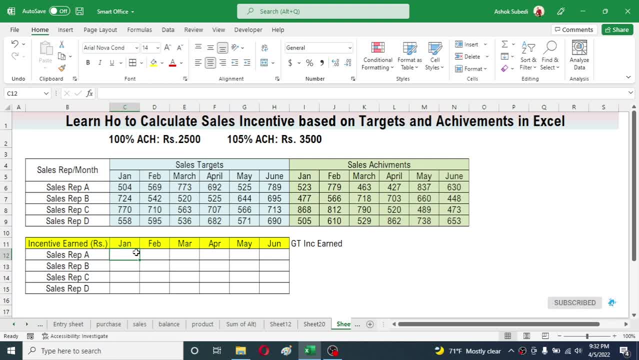 to combine multiple if formulas in one, which is also known as nested formula. so let's begin writing formula here in the first cell and we will directly copy this formula for all the remaining cells here. so first of all press equal to sign. then you start with writing a formula if. then 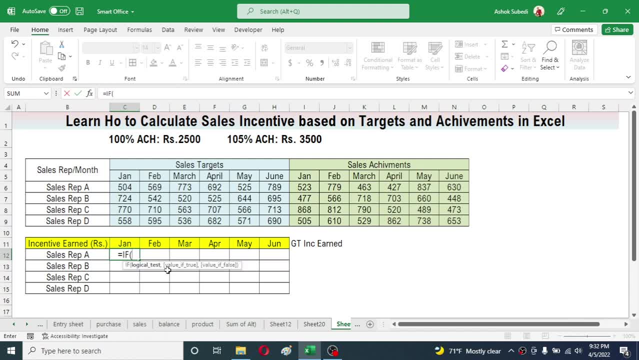 open bracket. now here we need to test our logic, and our first logic is: if the achievement percentage is greater than 105 percent, then the incentive is 3500. so first of all we need to test that, whether the achievement percentage is 105 percent or not- and to calculate the achievement percentage we 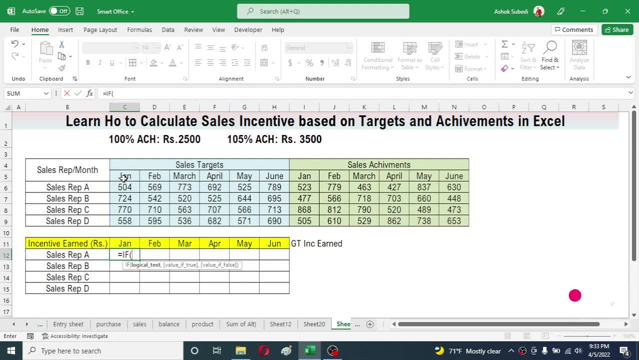 simply divide this sales target from the sales achievement. so here in this logical test, we need to click on this sales achievement, then divided by press the division sign, then click on the sales target of january month. in this way, now this formula will give us the achievement percentage. now, if the achievement percentage is greater than 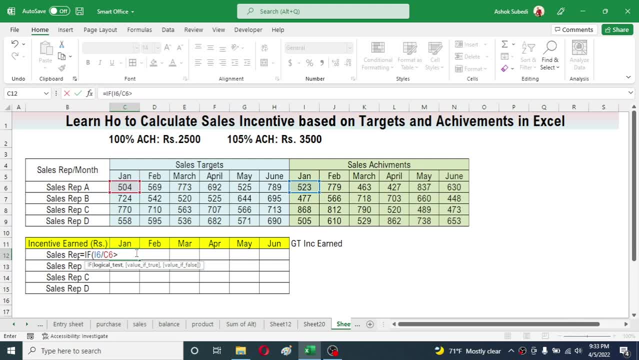 now type greater than, sign greater than or equal to. we have to type this greater than and equal to sign together here then press 105 percent percentage. so this is our logic. now give a comma and here in this value, if true, we need to write the value which we need to display here if this logic returns true. so in this case our 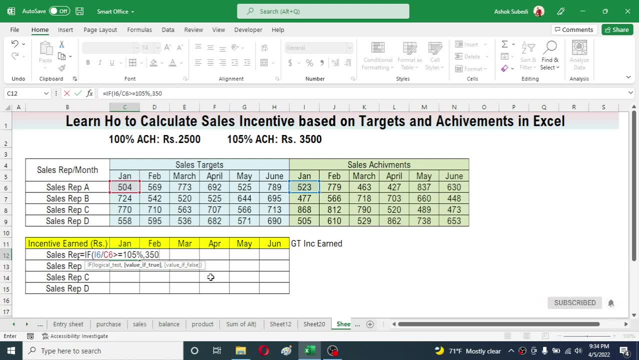 our value, if true, will be 3500 rupees. so we need to type 3500 here in this value. if true, now give a comma and here in this value, if false, we need to repeat the if formula again. so type if, then open bracket now here. we need to now test the second logic where the salesperson 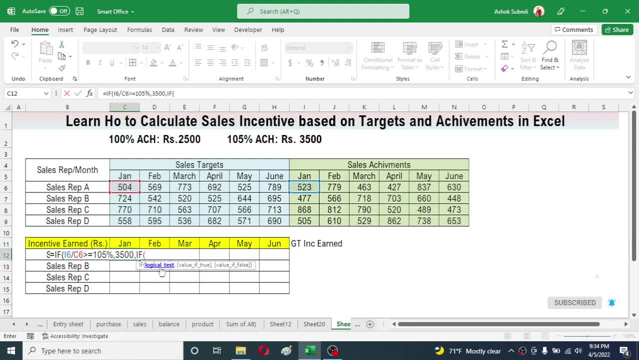 is applicable for 2500 rupees, which is the 100% achievement. so here we need to test the achievement percent: is 100% or not? so click on this sale divided by then, then click on the target of january and if this achievement percentage is greater than or equal to 100%, we need to. 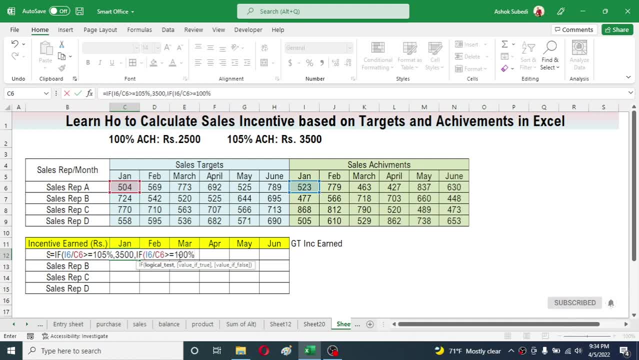 type greater than equal to, then 100%. now give a comma. and if this second logic returns true, then the salesperson is applicable or eligible for 2500 rupees incentive. so here we have to write 2500 in this value, if true, now give a comma. and here in this value, if false, if 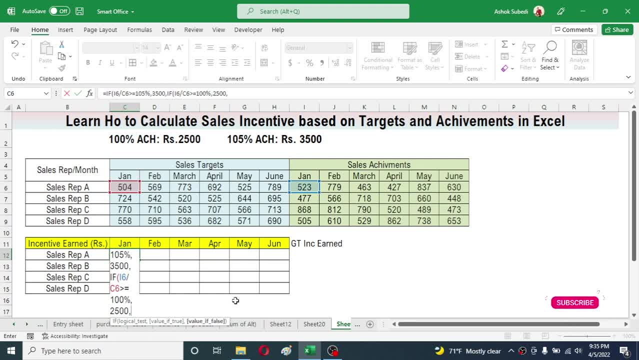 both the logic is not true, then in that case the salesperson is not eligible for any incentive. percent is 0 here in this case. so in the value, if false, simply type 0, then close the bracket, hit enter. now you here. we need to close one more bracket. that's why this error is given. 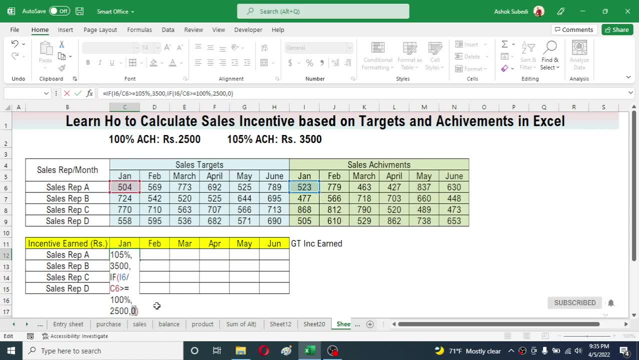 so formula and closing one more bracket here, closing one more bracket, then hit enter. now here you can see the incentive amount is calculated as 2500. if you see the achievement of january month. if you check from here this value divided by this value, then the achievement percentage: 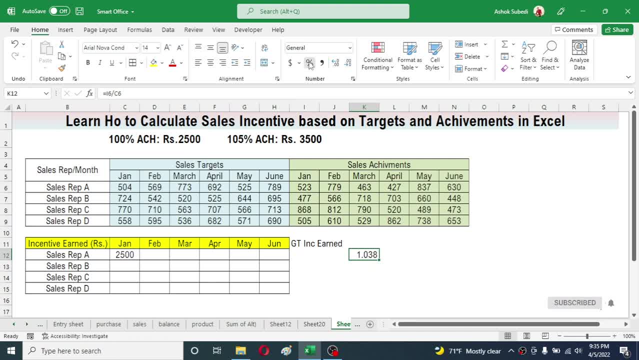 here is 100.3 percent, 104 percent, which is greater than 100 percent, and the eligible or applicable incentive amount is 2500, which is calculated here. now. you can simply drag this formula till the last month, and you can also drag this formula for other sales persons.